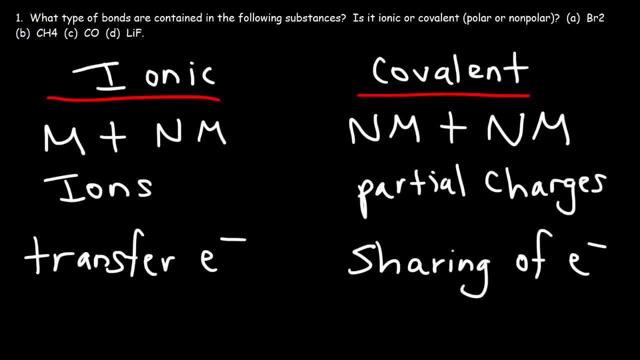 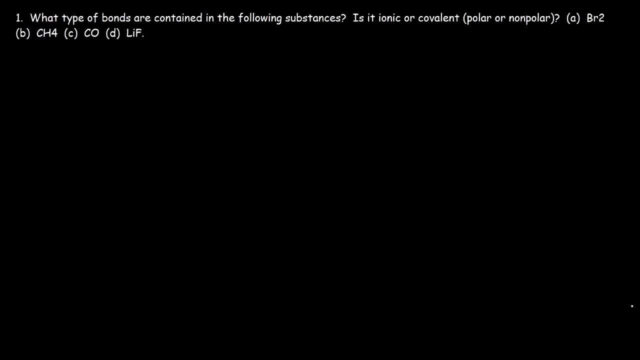 But let's see if we have enough information to answer this particular question. So let's understand part A, Or let's answer it: Br2.. What type of bonds are contained in that substance? So Br2 is bromine And it looks like this: 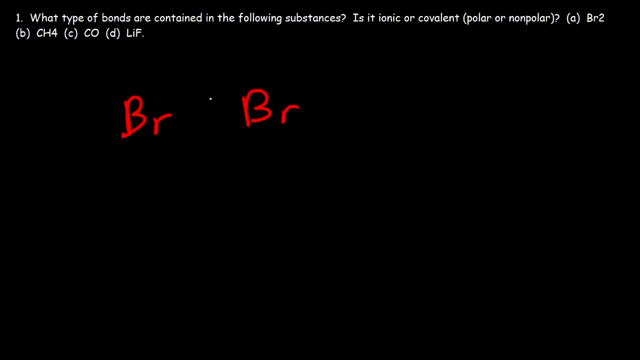 So you have a molecule which is composed of multiple atoms- In this case this molecule has two atoms- And within this molecule you have a single bond And each atom has three lone pairs. So that's how the bromine molecule looks like. 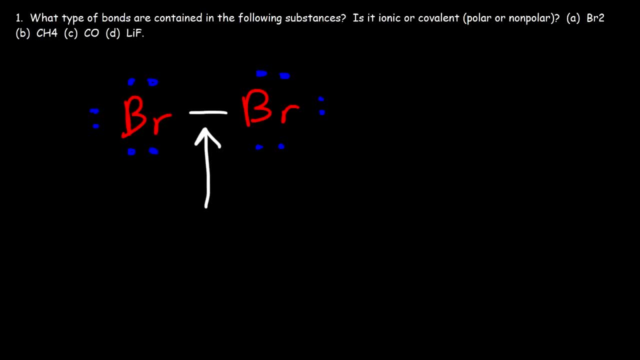 But now let's describe the bond that holds. holds these two atoms together? Is it ionic or covalent? So do we have two non-metals, Or is this a metal mixed with a non-metal? Well, you need to know where the metals and the non-metals are located. 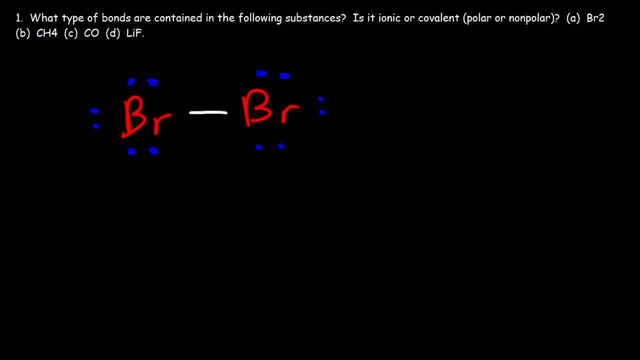 in the periodic table to answer that question in the first place, And so let's take a minute and talk about that. So if you go and get your periodic table, or if you don't have one, go to Google Images and look for the following table: 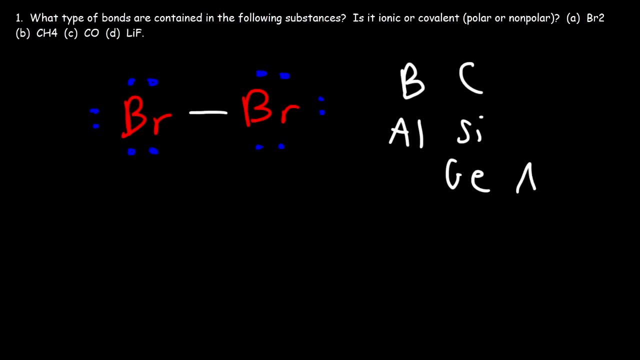 It's called elements. They should be in the upper right side of the periodic table And you're going to see this line that divides some of these elements. Now, most of the elements located near that line are known as metalloids or semiconductors. 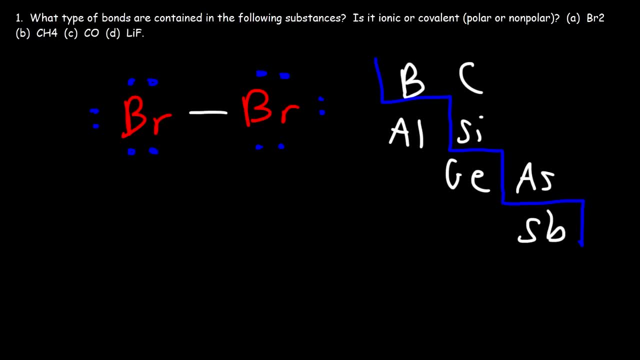 A metalloid has properties that are in between a metal and a non-metal, But what you want to take from this is that the non-metals are located to the right of that line And to the left of that line you have the metals. 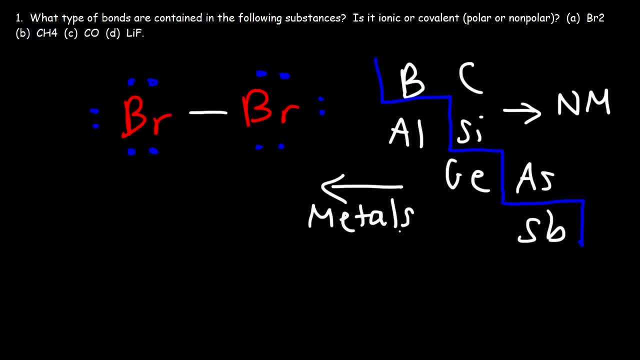 So by using the periodic table, you can quickly determine if an element is considered a metal, a non-metal, or if it's, on a line, a metalloid. So bromine is on the right side of the periodic table. Therefore, bromine is considered a non-metal. 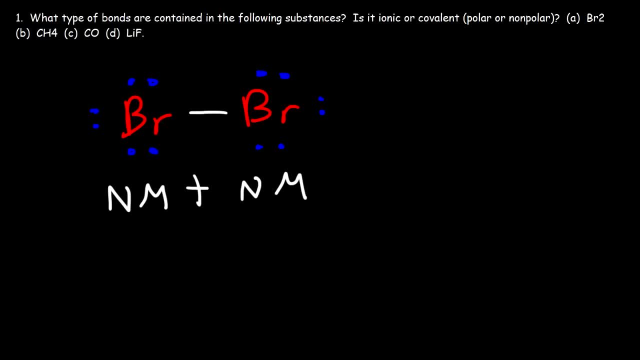 So here we have two non-metals mixed together, And because those elements are the same, the two electrons that are in this bond will be shared equally between those two atoms, And so we're going to have a covalent bond. So anytime there's some sort of sharing of electrons, 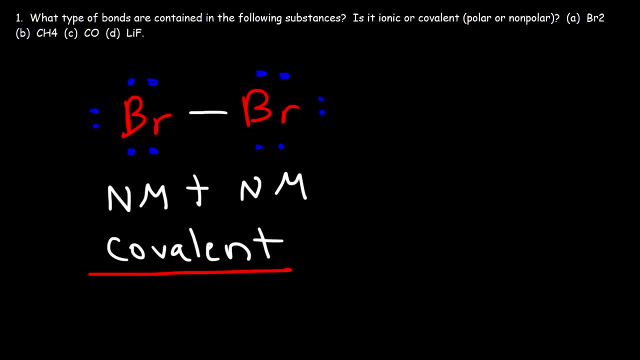 you have a covalent bond. Now that we have a covalent bond, we need to discuss: is it a polar covalent bond or is it a non-polar covalent bond? In a non-polar covalent bond, the electrons are shared equally. 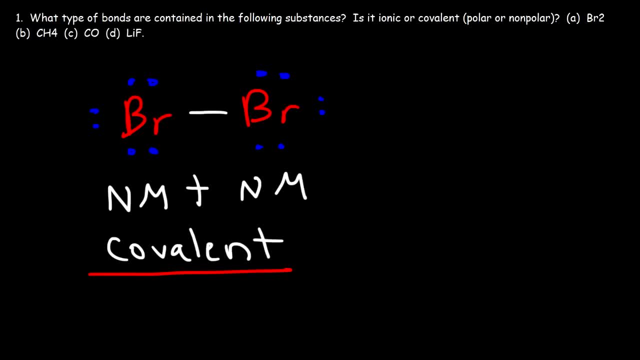 If it's polar covalent, that means that the electrons are being shared between the two atoms, but relatively unequally. So in this case, this is going to be a non-polar covalent bond, because the elements are the same. 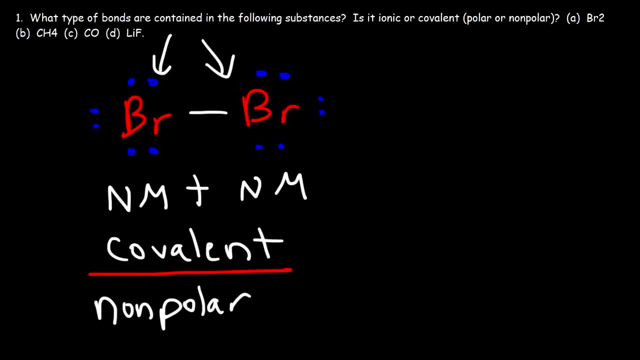 In order for it to be a polar covalent bond, the elements have to be different. So let me just give you some notes on this. So if it's going to be polar covalent, the electronegativity difference has to be 0.5 or more. 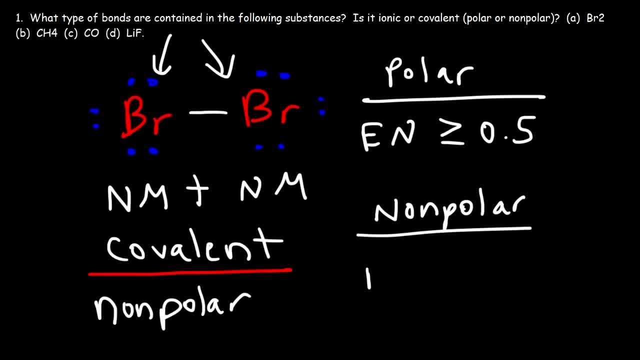 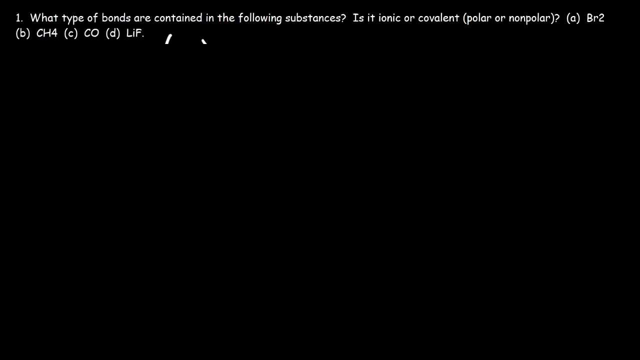 A non-polar covalent bond has an electronegativity difference value of 0.4 or less, So just keep that in mind. Now let's consider methane, CH4.. Here's the Lewis structure of methane, And we're going to focus on the carbon-hydrogen bond. 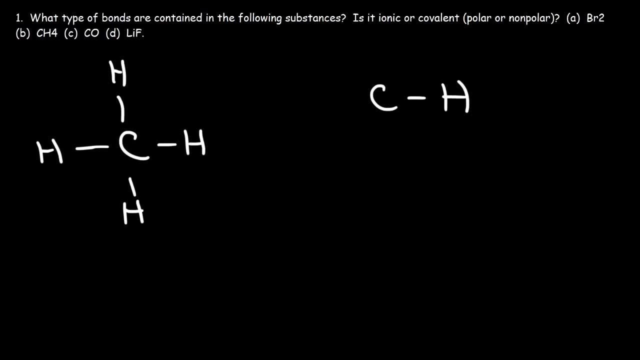 So this particular bond, is it ionic or is it covalent? What would you say? And let's compare that bond with the bond between two hydrogen atoms. Now, automatically, if the elements are the same in a chemical bond, then you know it's going to be a non-polar covalent bond. 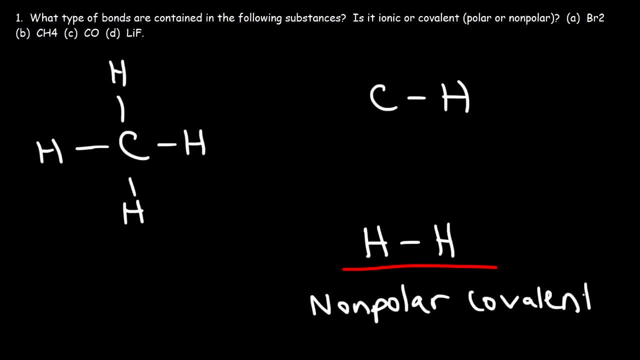 But if the elements are different, it could be ionic or it could be polar covalent, Or it could be even non-polar covalent. But first let's see if it's ionic or covalent. So carbon, is it a metal or is it a non-metal? 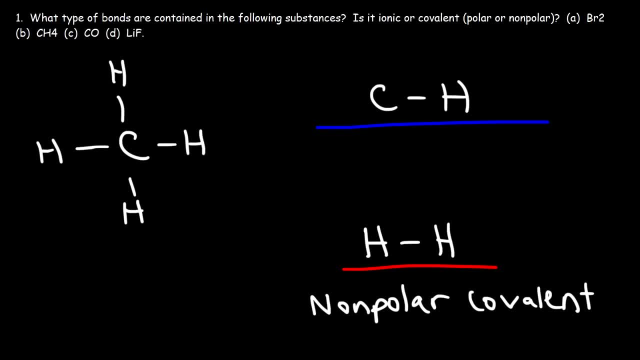 What would you say? Carbon is considered to be a non-metal. It's on the right side of that line- Hydrogen. even though it's on the left side, it's not really considered to be a metal. It's considered to be a non-metal. 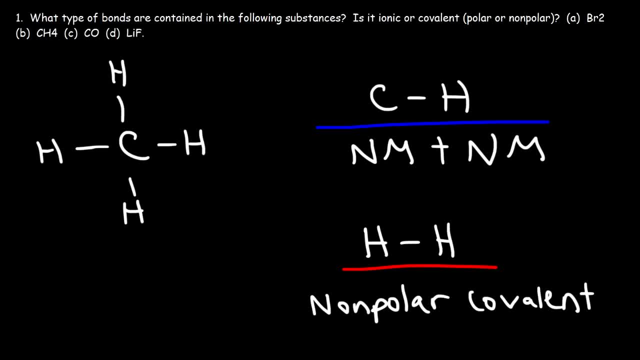 So be careful with that one. So here we have two non-metals combined. So therefore we know that this is a covalent bond. Now is it polar covalent or is it non-polar covalent? To answer that, because the atoms in that bond are different. 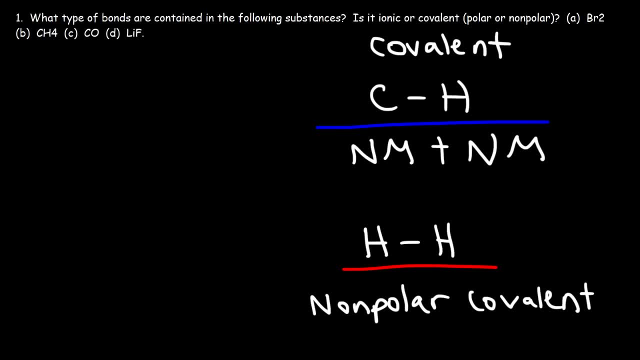 we need to look at the electronegatives, The electronegativity values. Here are some common values that you want to be familiar with. The electronegativity value for hydrogen is 2.1.. For boron it's 2.0.. 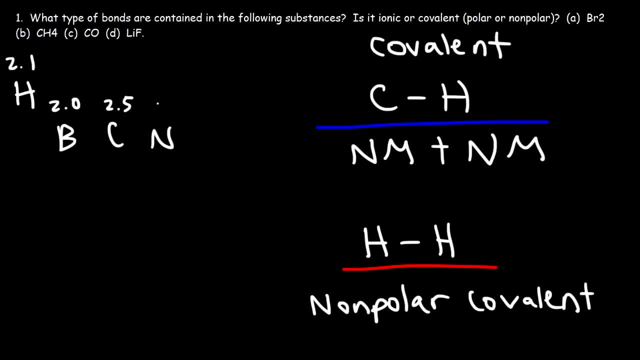 For carbon 2.5.. Nitrogen is 3.0.. And then oxygen is 3.5.. Fluorine is 4.0.. It's the highest, And then we have chlorine, which is 3.0.. 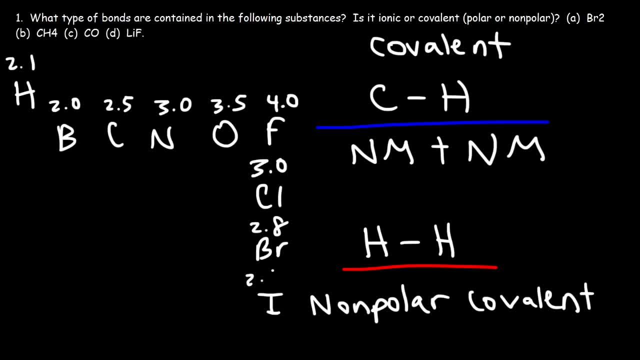 Bromine 2.8.. Iodine 2.5.. And you can look up these values if you go to Google Images and type in electronegativity values, It should come up, So in the C-H bond. the electronegativity difference between the two elements is 2.5 minus 2.1, which is 0.4.. So therefore, the bond is considered to be non-polar. If the elements are the same, then the E-N difference will be 0.. 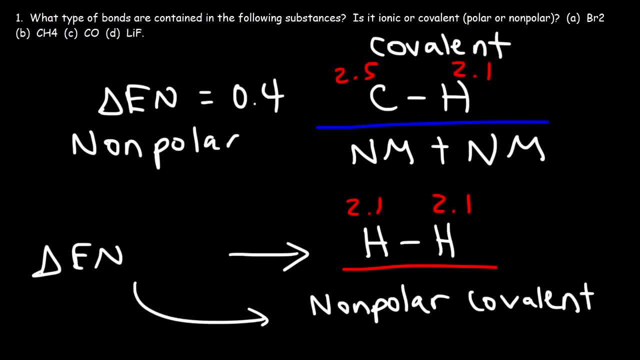 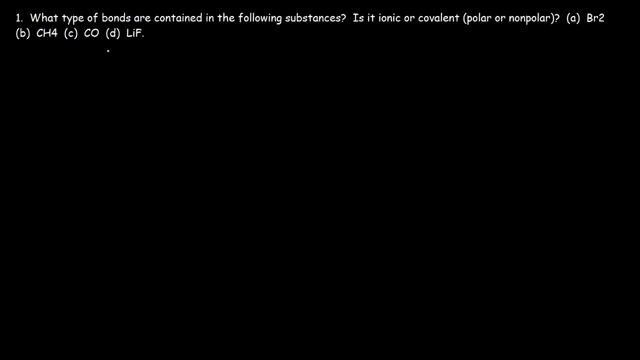 Which means it's definitely non-polar. So both of these bonds are non-polar, covalent bonds. Now let's move on to Part C. So what type of bond do we have between the elements carbon and oxygen? What would you say? Is it ionic or is it covalent? 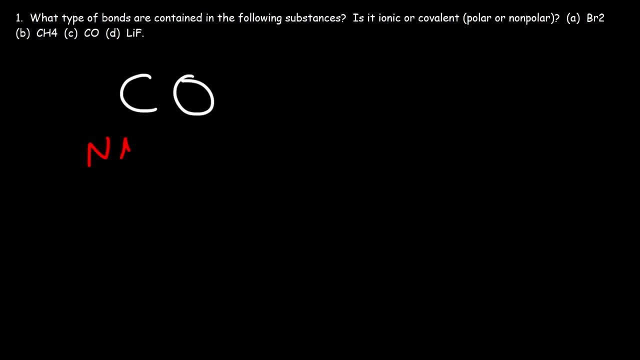 Well, carbon is a non-metal and oxygen is a non-metal. So we have two non-metals, which means that the bond in between them is covalent rather than ionic. Now to determine if it's polar or non-polar. we need to look at the electronegativity values. Carbon has an E-N value of 2.5 and oxygen is 3.5.. So the electronegativity difference between the two elements is 1.0, which is greater than 0.5.. 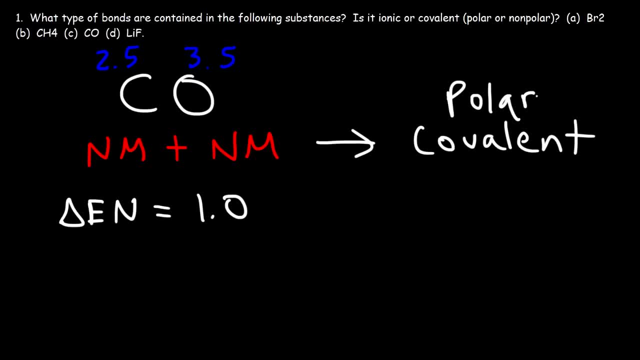 So, therefore, this particular bond is a polar covalent bond, And that's basically it. That's how you can quickly tell if it's polar covalent or non-polar covalent, And it's by looking at the E-N difference values. 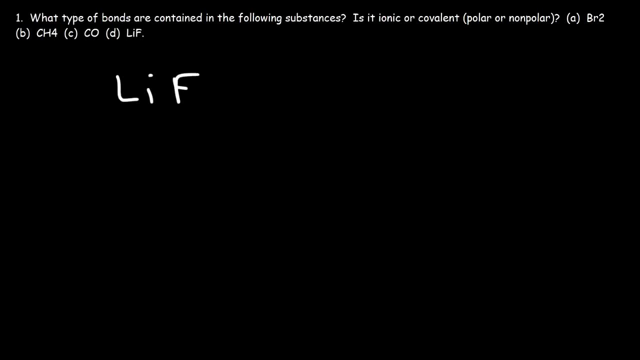 Now let's move on to lithium fluoride. Is it ionic or is it covalent? Well, lithium is on the left side of the periodic table, so it's a metal. In fact, it's an alkali metal. Fluorine is on the right side of the table. 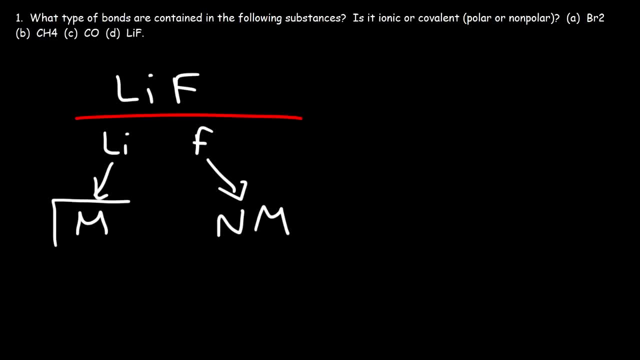 It's a halogen, which is a type of non-metal, And so here we have a metal and a non-metal. When you see that, that tells you that you're dealing with an ionic bond. Now let's go deeper into ionic and covalent bonds. 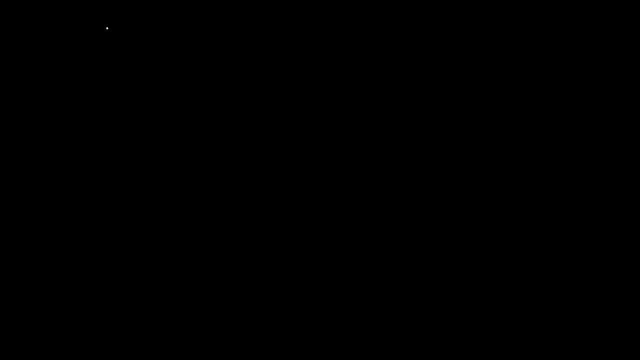 Let's understand how they're made. Now let's start with ionic bonds before we go back into covalent bonds. Lithium, as an atom, has one valence electron. Fluorine, as an atom, has seven valence electrons. 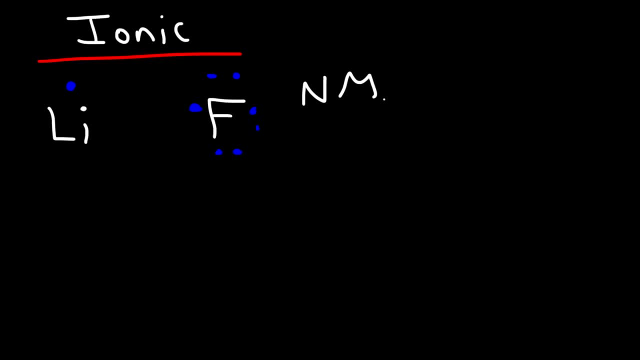 Fluorine, as a non-metal, has a very high electronegativity value: It's 4.0.. And lithium, as a metal, has a very low electronegativity value, which I don't remember what the number is. 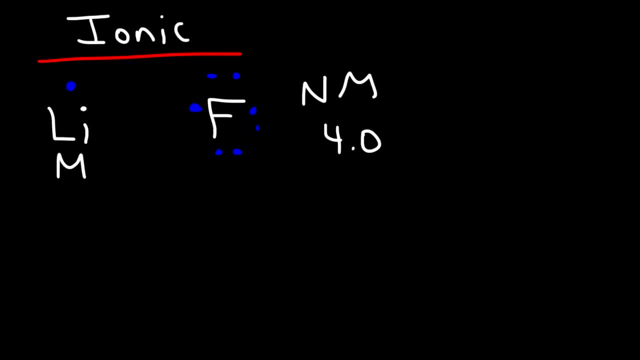 but it might be like 1.0 or less, But it's pretty low And because fluorine is more electronegative, it has a strong affinity for electrons. It really wants it. And the halogens: they like to have eight electrons. 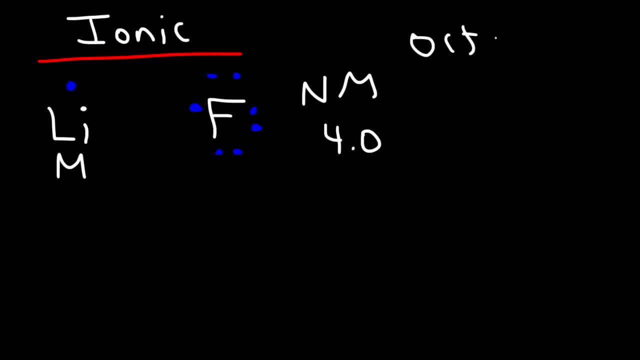 to satisfy the octet requirement. They want eight electrons in their outer energy level to be stable, to be satisfied, And so what you need to understand is that metals they like to give up electrons, Non-metals like to take them. 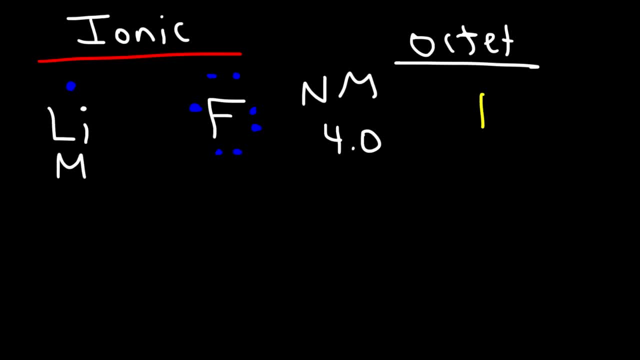 So what's going to happen here is we're going to have a transfer of electrons, So lithium is going to give up its one electron to fluorine, And so when lithium loses that one electron, it's going to acquire a positive charge When fluorine gains that electron. 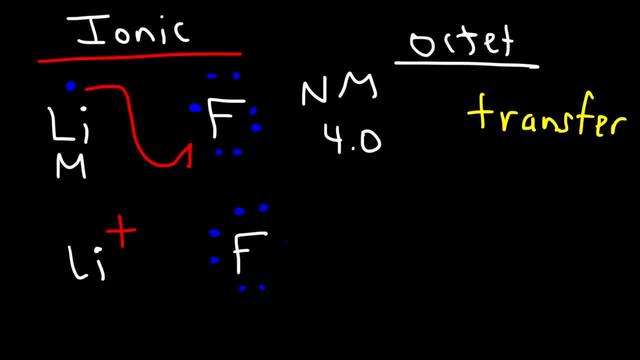 it acquires a negative charge. Now, what do you know about opposite charges? If you have a positive charge next to, let's say, a negative charge, what will the two do? Well, opposite charges attract, And so you're going to have a force of attraction. 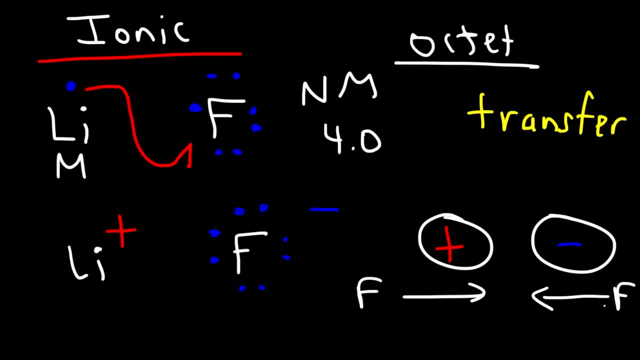 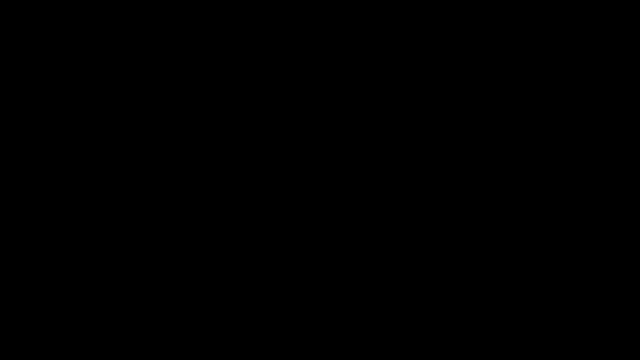 And this force keeps them together. So this is the chemical bond between these two ions. It's called an ionic bond, So that electrostatic force of attraction is what holds the ionic bonds together. Now let's consider this situation in a covalent bond. 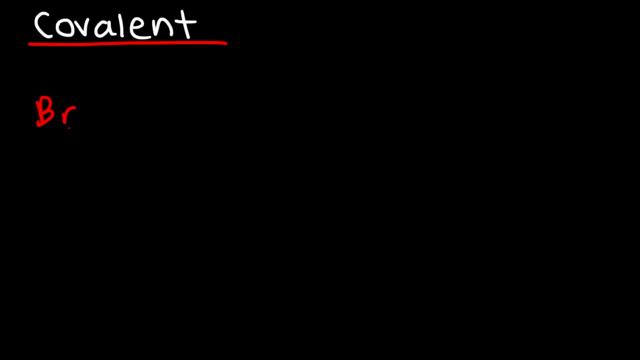 And let's use bromine as an example. So bromine as an atom has seven valence electrons, like fluorine, And because they're in the same column, group 7a of the periodic table, they're both halogens And, as a result, 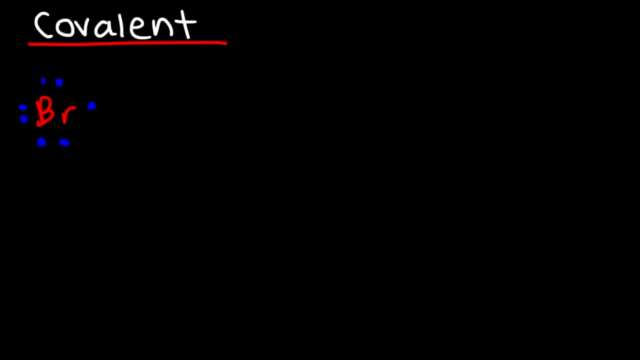 they both want to be covalent: Eight electrons. So when a bromine atom meets up with, let's say, another bromine atom, both of them, they want to have eight electrons, but none of them want to give up their electrons. 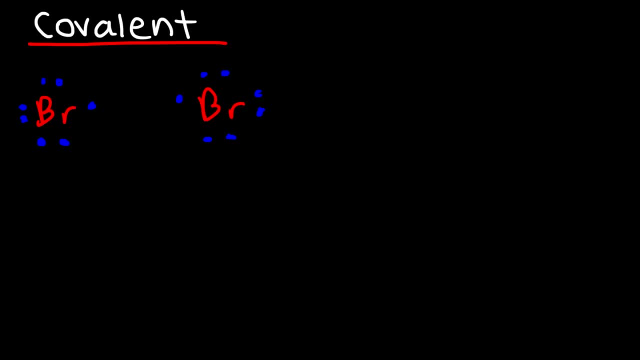 And so they're like: how are we going to figure out this situation? I need an extra electron and you need an extra electron. What sort of deal can we make so that we both get what we want? In this case, what they do is: 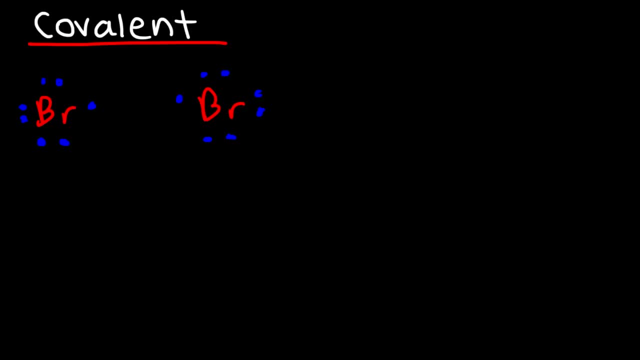 they share electrons, And so bromine. it gives up one electron to form a bond, and the other, bromine atom, gives up one electron as well. And keep in mind, it takes two electrons to make a bond, And so we get the bromine molecule. 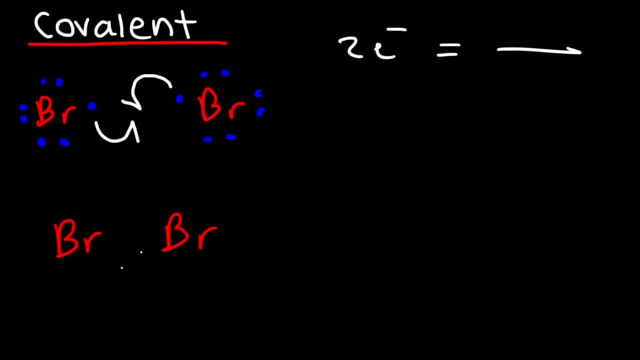 which looks like this, And there's a single bond between them. So each bromine atom now has eight electrons around it. So if you look at the bromine atom on the left, two, four, six and this is considered two. 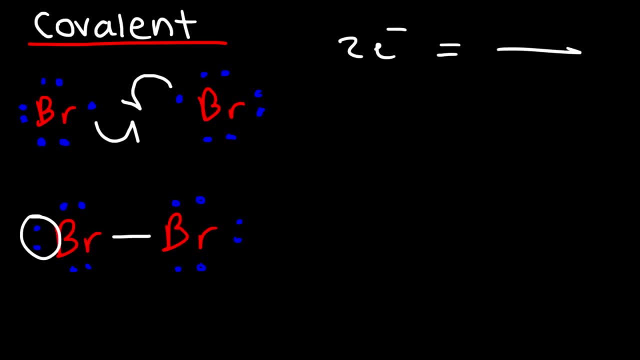 so that's eight electrons. The same is true for the one on the right: It has two, four, six and the two shared electrons, so it has eight, And in this arrangement they satisfy the octet requirement that they have. 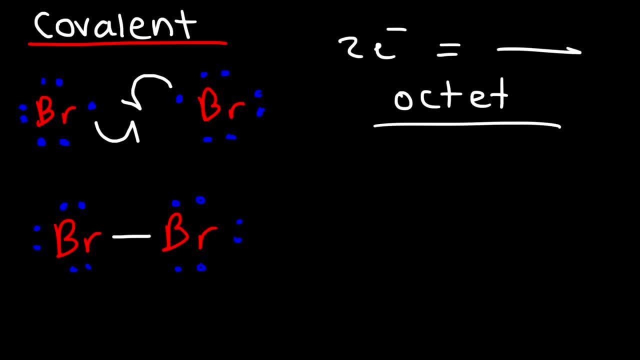 That is, to have eight electrons in their outermost energy level. Now, because the electronegativity of the two atoms in this molecule is the same, the electrons are shared equally, and so this is going to be a nonpolar covalent bond. 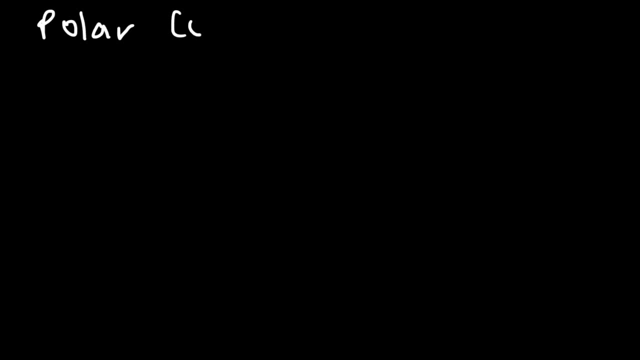 Now let's talk about the other situation, a polar covalent bond, And in this video we use the example of carbon and oxygen. So carbon, as an atom, has four valence electrons. Oxygen, as an atom, has six valence electrons. 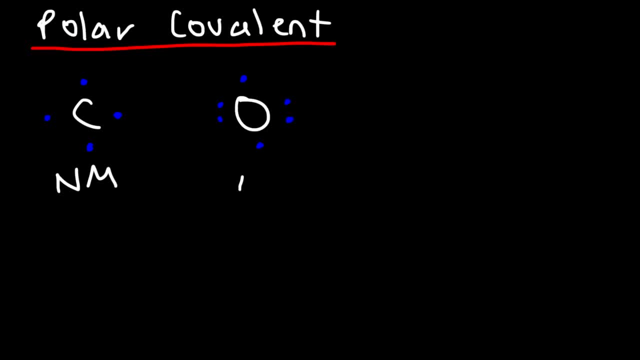 Now, both of these are nonmetals and, as a result, they want to acquire electrons. So, like in the previous example, they need to make a deal, They need to share electrons so that both of them can have eight. The question is: 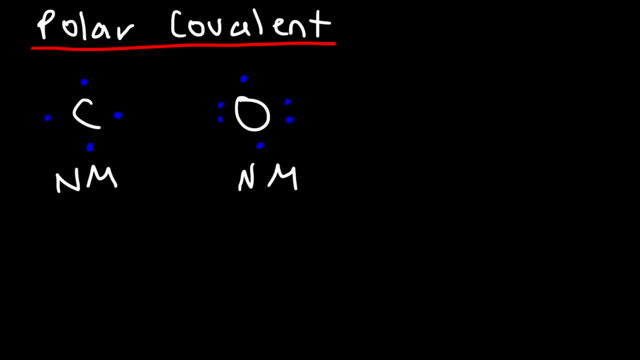 how are they going to do it? In this case, they're going to share electrons unequally. For this to work, carbon is going to give two electrons to make a bond between carbon and oxygen, But oxygen is going to give four electrons. 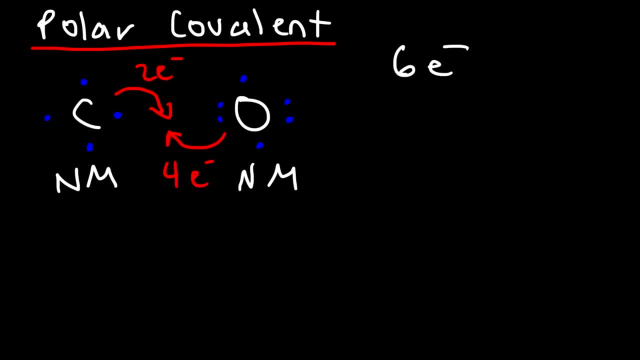 And so we have a total of six shared electrons and, if you recall, it takes two shared electrons to make one bond. So six electrons will make a triple bond. The Lewis structure between carbon and oxygen it looks like this. So those are the six electrons. 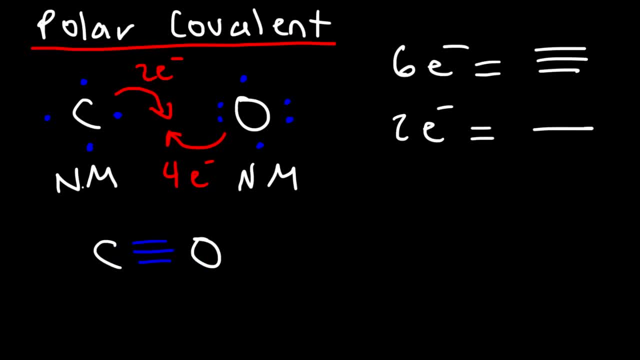 that were used to make that bond. So carbon gave up two, which means that it has two electrons left. Oxygen: it gave up four, which means it also has two left. And so this is the Lewis structure for carbon monoxide. Carbon has an electronegativity value of 2.5,. 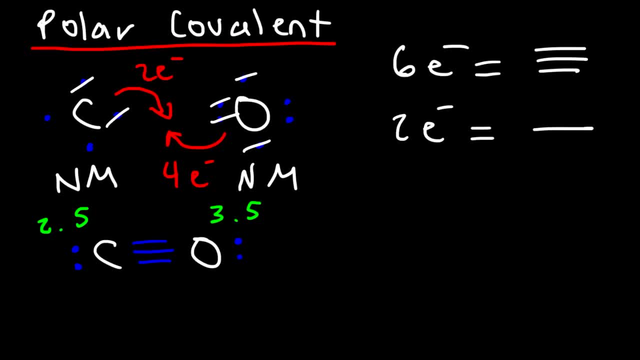 and for oxygen it's 3.5. And because oxygen is more electronegative than carbon, it's going to pull the electrons in that bond closer to itself. So oxygen will acquire a partial negative charge, And so you have this delta-looking symbol. 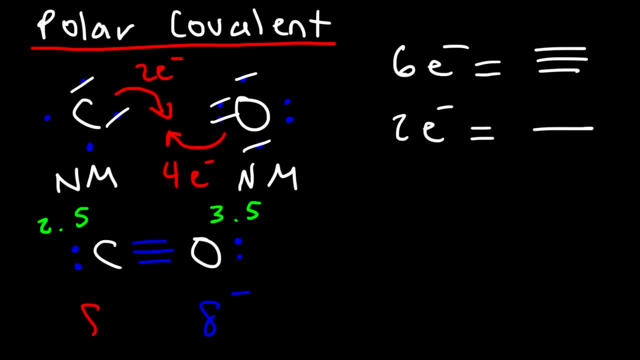 for partial charges And carbon. because it has a lower electronegativity value relative to oxygen. it's going to be losing some electrons to oxygen. Oxygen is going to pull those electrons more closer to itself. Both of them are still sharing electrons. 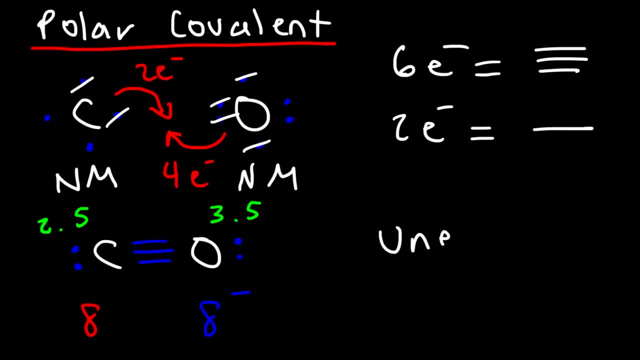 but what we have is an unequal sharing of electrons And, due to this unequal sharing, one element pulls on the electrons more than the other one does, And because oxygen has a greater pull, it's going to have a partial negative charge, whereas carbon is going to have. 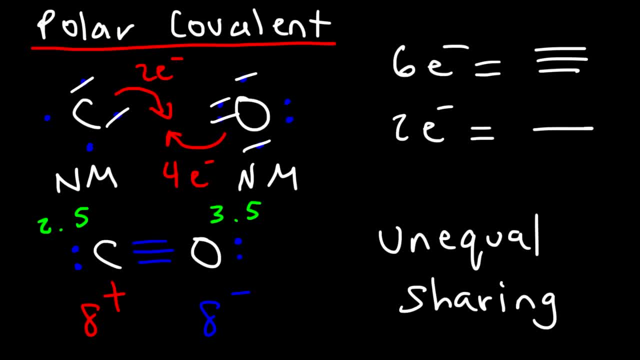 a partial positive charge, And when you have these partial charges in a covalent bond, it makes it a polar covalent bond. When something is polar, it means that it's still neutral overall, but it's polarized. One side has a partial positive charge. 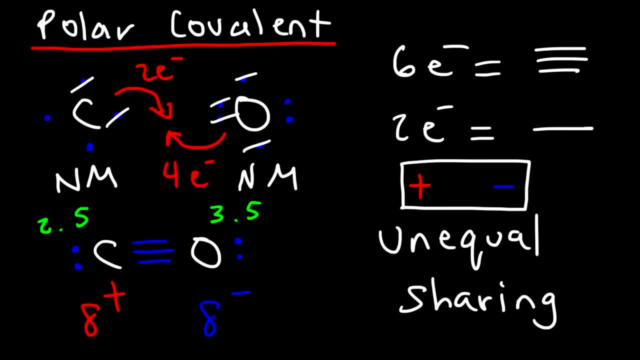 and the other side has a partial negative charge, And that's what it means for something to be polarized. You have a separation of charges in something that is intrinsically neutral, Because overall this is a neutral molecule If you add plus one and negative one. 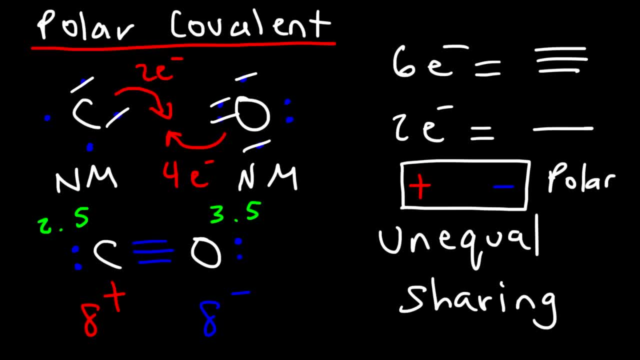 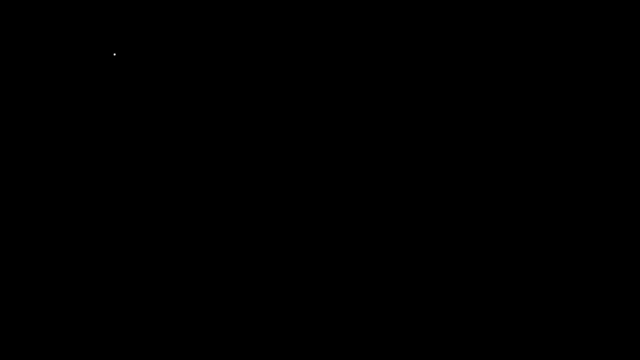 you get zero, But you have a spread of partial charges within this individual molecule, And so this is a polar covalent bond. So what I'm going to do now is make a summary of what we've just considered. So we talked about ionic bonds. 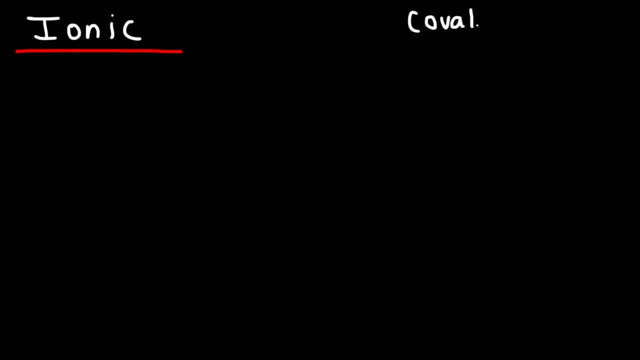 and we talked about covalent bonds. Now, within a covalent bond, you can have two types: It can be a polar covalent bond or you can have a nonpolar covalent bond. So for the ionic bond, 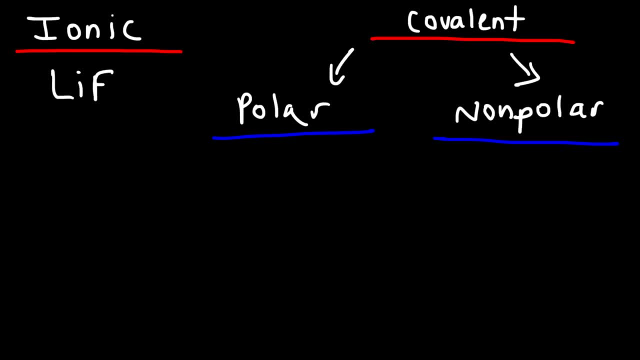 we have the example of lithium fluoride. Now, in an ionic bond you have ions. Lithium has a positive charge, Fluorine has a negative charge. In a polar covalent bond we had molecules like carbon monoxide. 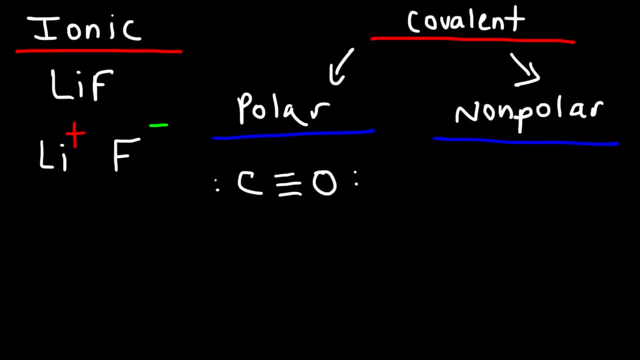 However, we didn't have a full charge, but we had a partial charge. Carbon was partially positive and oxygen was partially negative. So make sure you see the difference In ionic bonds. you have full charges like a plus one or a minus one. 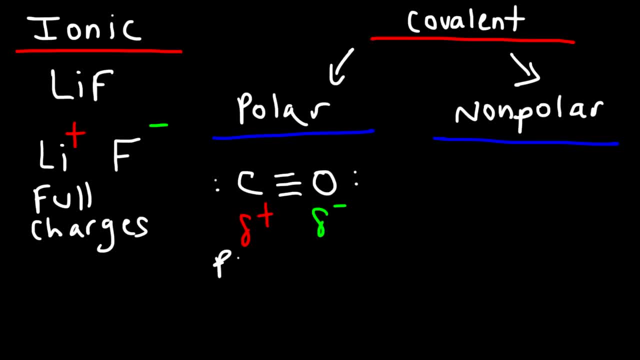 Whereas in a polar covalent bond you may have partial charges- They could be 0.1, 0.2, but it's not a full charge In a nonpolar covalent bond, as in the case of the bromine molecule. 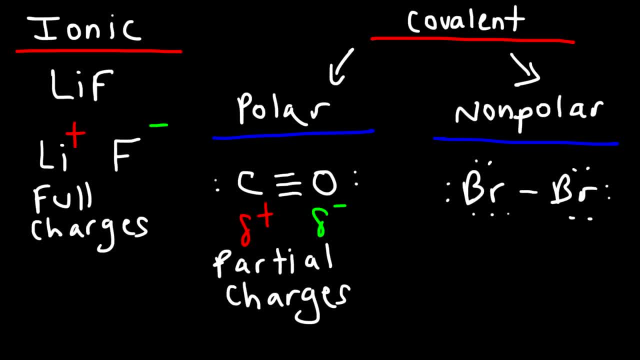 the electrons in this molecule are shared equally, and so there are no partial charges. And, if you recall, ionic bonds are typically made up of metals and nonmetals, Whereas covalent bonds, they, typically consist of two nonmetals. 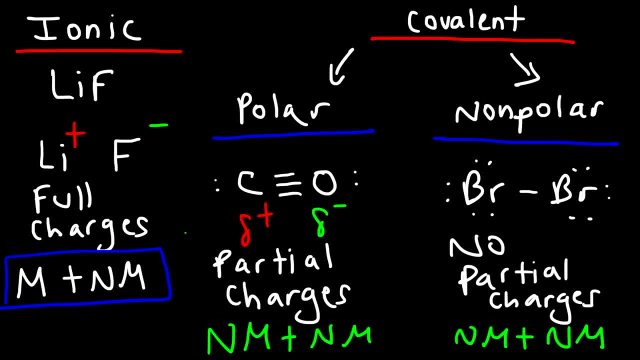 be it polar covalent or nonpolar covalent. And remember the EN difference for a polar covalent bond has to be 0.5 or more. For a nonpolar covalent bond, it's usually 0.4 or less. 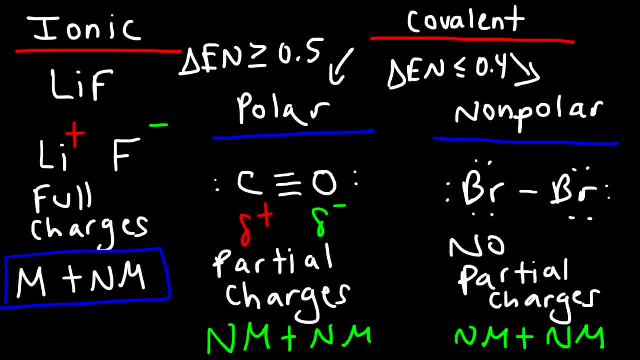 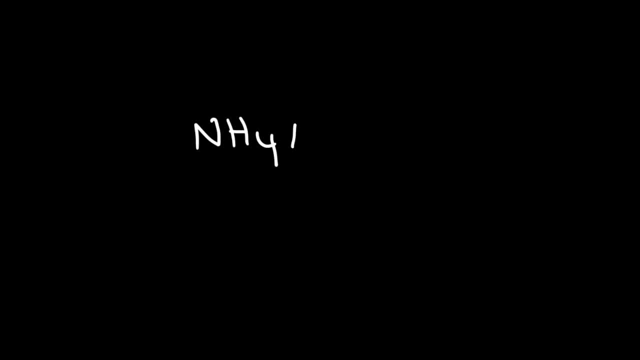 So that's basically it for this video. That's a summary sheet of what I have, And there's one more thing I do want to mention: Ammonium nitrate. This is one of those exceptions you need to watch out for. Would you consider it to be ionic or covalent? 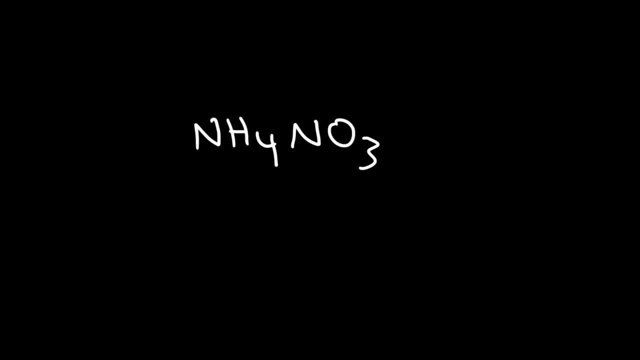 Now looking at the elements nitrogen, hydrogen and oxygen, you'll probably notice that there are no metals in this example, So you might be thinking this is a situation between two nonmetals, which it is. However, it's not. 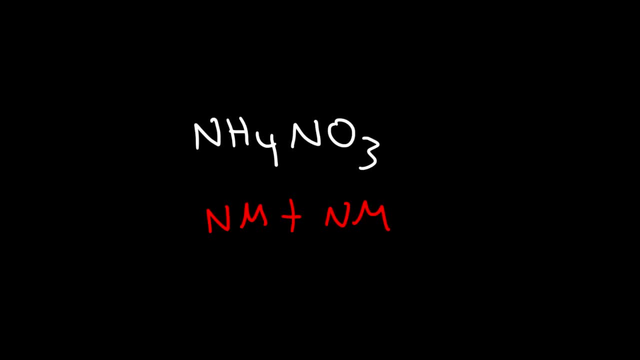 You can't rule out ionic bonds in this case, Because it turns out that this compound has a mixture of ionic and covalent bonds. Ammonium is a polyatomic ion with a positive charge And nitrate is a polyatomic ion. 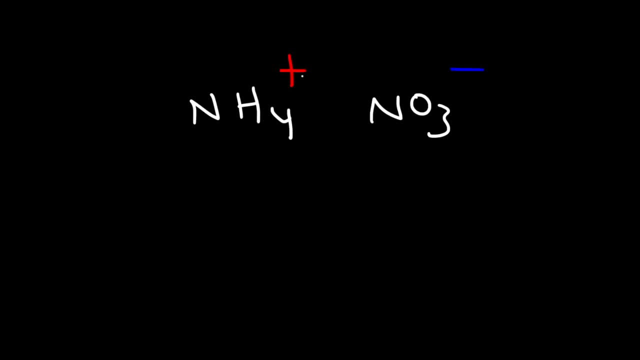 with negative charges. So between the ammonium ions and the nitrate ions you do have an ionic bond, Even though there's no metals. So this is one of those exceptions where you have an ionic bond between two nonmetals. 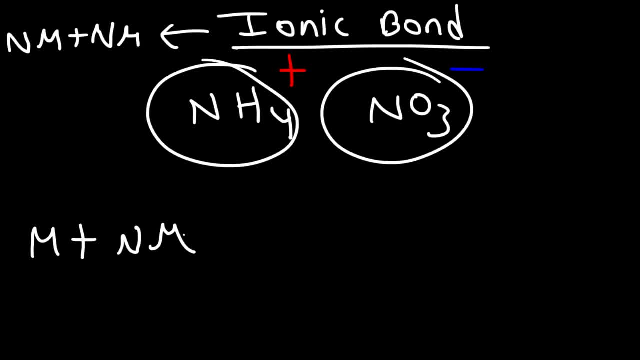 So when you see a metal and a nonmetal, that's typically an ionic bond. If you see two nonmetals, usually it's a covalent bond, But it could be an exception, as you see in this case. Now for this particular substance.